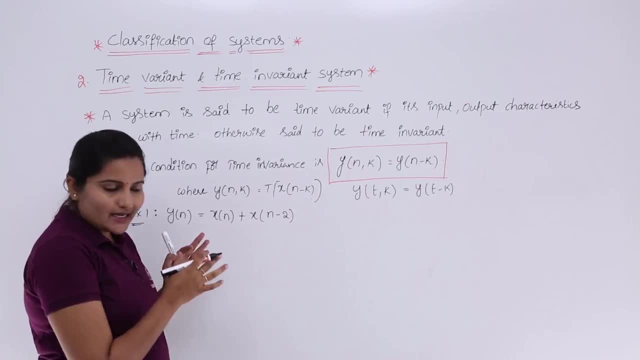 if you are having. This is a system with a response y of n equal to x of n plus x of n minus 2.. First of all you need to calculate y of n comma k. So y of n comma k is nothing but t of. that means transform of x of n minus. 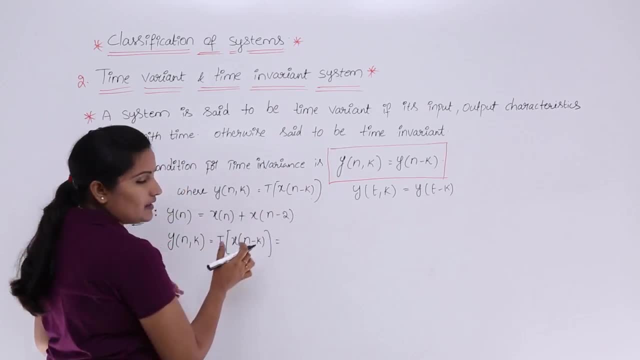 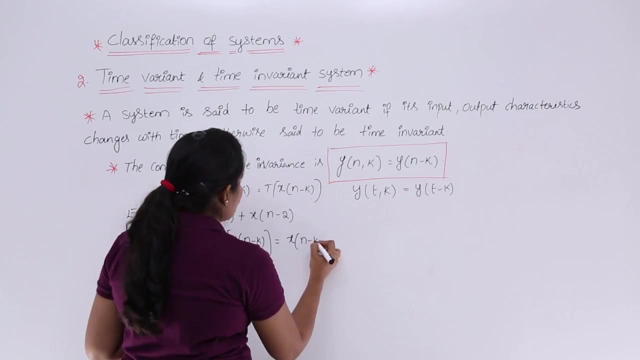 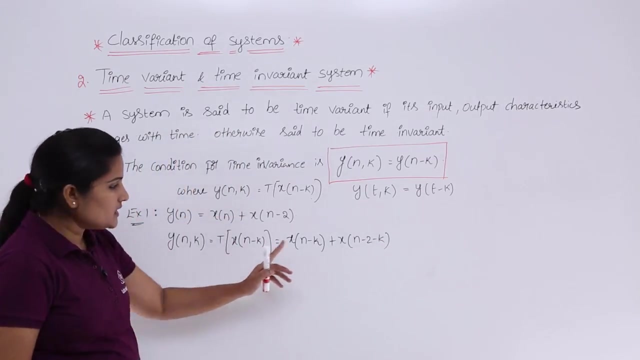 k, that means you need to delay each x signal with k samples. So that means: so this is equivalent to x of n minus k plus x of n minus 2 minus k. so like this you need to write: so that means you need to delay by k samples. 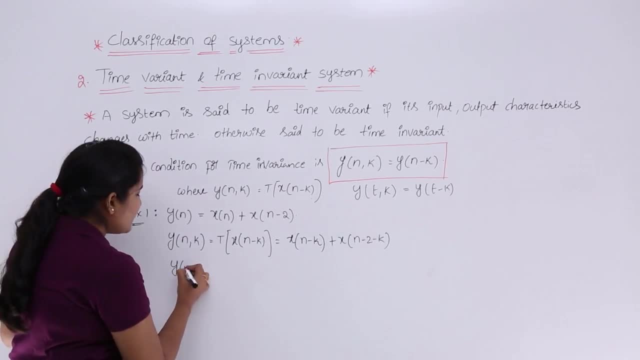 so now I am writing y of n minus k. so now here this is nothing, but just by substituting the value in the response. this is the value. so here this is just delaying your x signal with k samples. this is substituting the value in the response directly. so here y of n minus k is equivalent to: 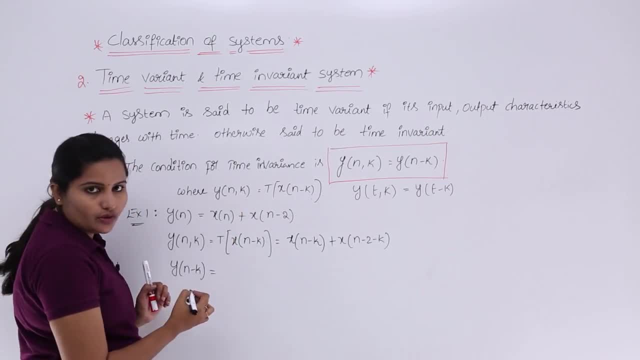 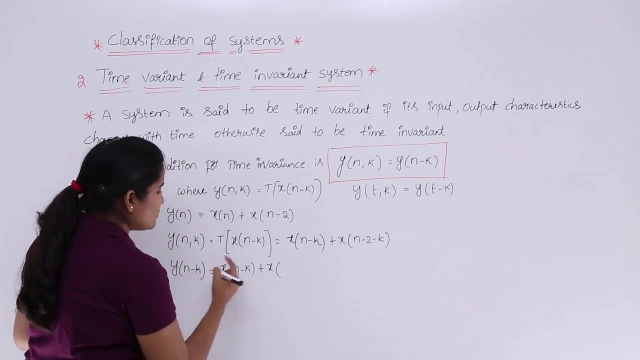 here, wherever you are having n there, you need to substitute n minus k. so x of n minus k plus x of in place of n you need to substitute n minus k minus 2. so if you observe these two, then so here y of n comma k is equivalent to y of n minus k. 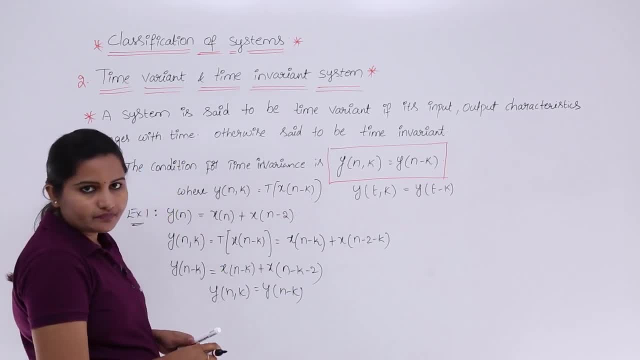 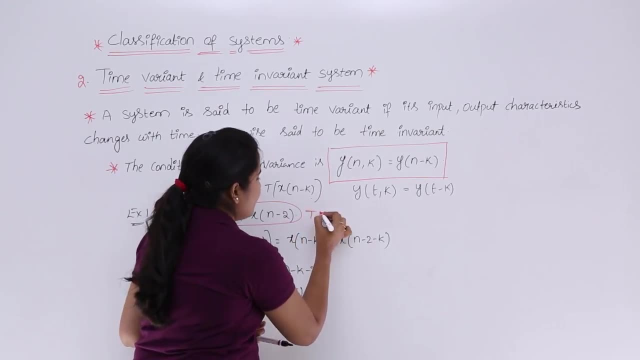 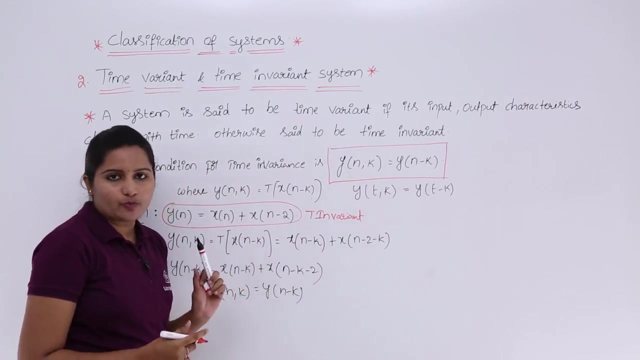 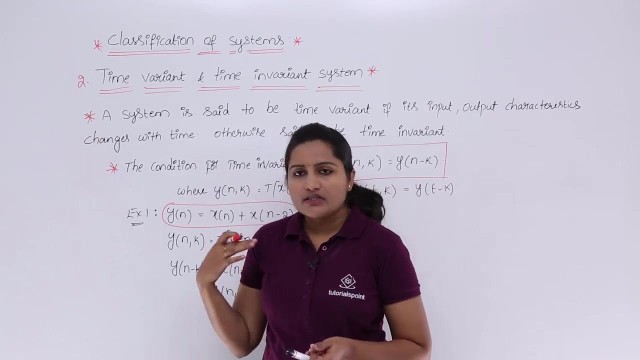 so this is going to satisfy this condition. so this system, with this response, is said to be time invariant. so this is time invariant system response. by observing the response itself, we can say which type of system that is. that means time variant system or time invariant system. so by observing the response itself, we said: this is it? 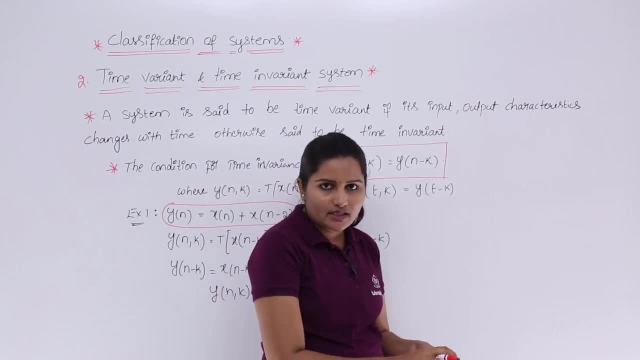 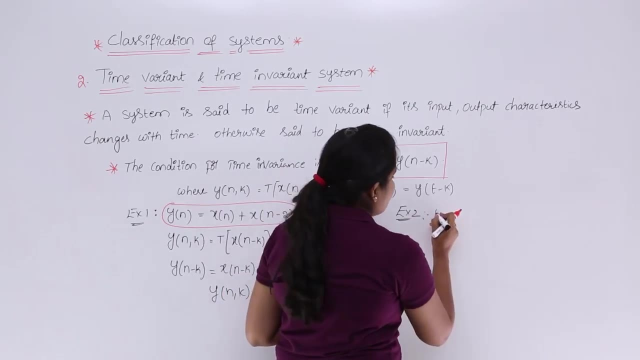 time invariant system, for example. any other system is given. that means I am considering some other example for this. if a system is given, so with response, y of n is equal to x of n. this time they given like this, n into x of n minus 3. like this they given x of n plus n into 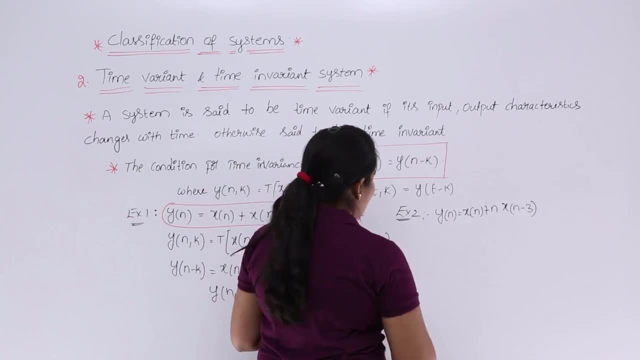 x of n minus 3 they given. so now, first of all to check time variant and invariant. you need to consider your input time variant and invariant. you need to consider your input time variant. and here, if at x the same function is given with constant x, that is, of n comma k, x will give. 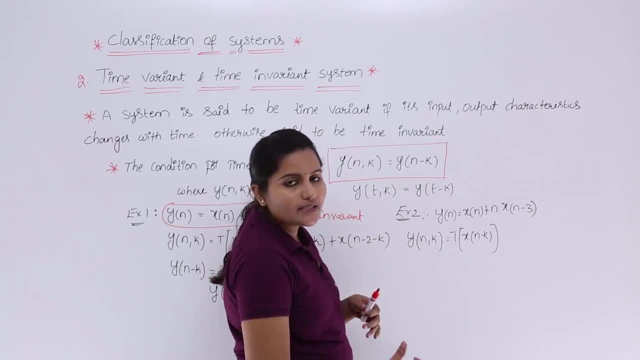 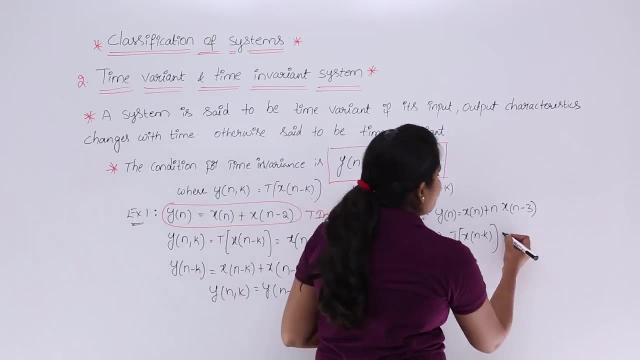 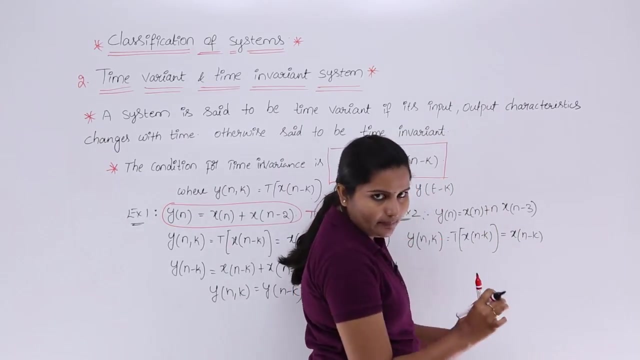 as o u x zoom out, this might showейств 1950 of x is equal to 1 over 0.. Ok, I will consider any. either case you must. if is x times x is equal to. or will I calculate it here you have to. Here I am writing at x as n comma k. so that means input change mean transform of x of n minus k. you need to delay your Xsignal with K samples. each time that is a shifted version of X or normal version of X, you need to delay k samples. so that means: so here I am delaying k samples. 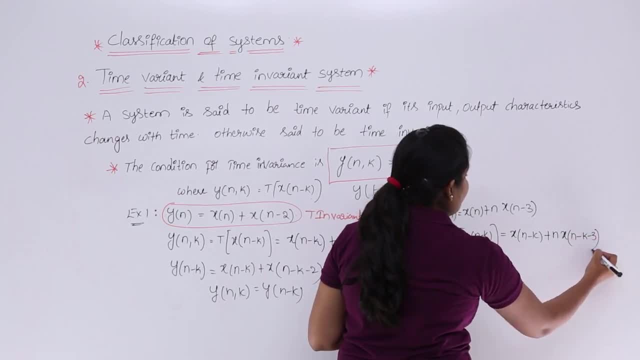 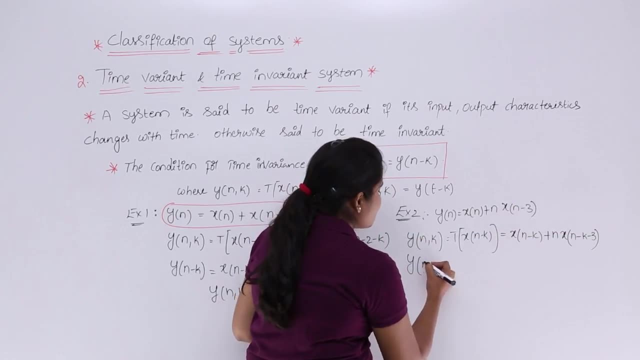 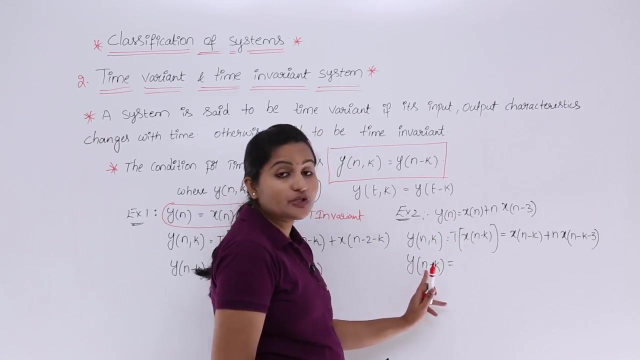 So n minus k samples. you need to delay. that means n minus 3 minus k also. you can write: So here now you need to check for y of n minus k. this is nothing. but wherever you are having n value there, you need to substitute n minus k value. that is the meaning. 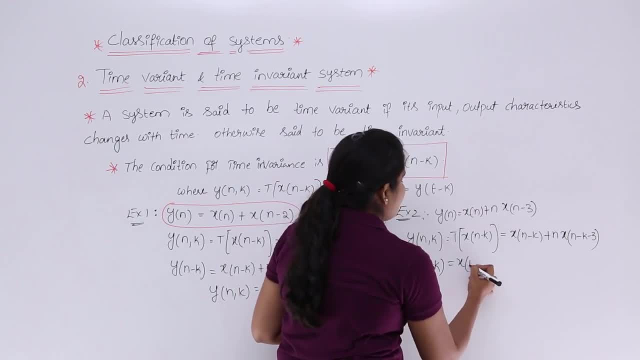 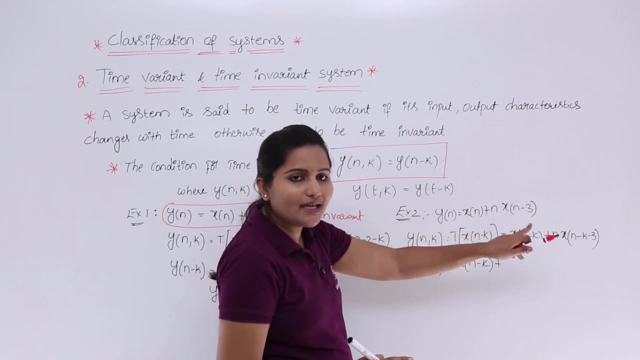 So now, here you are having n value. so that is why I am substituting n minus, k plus. here also, you are having n value. so here- this is the meaning- you need to delay x signal. wherever signal you are having, there you need to delay, but here, this is the meaning where you are. 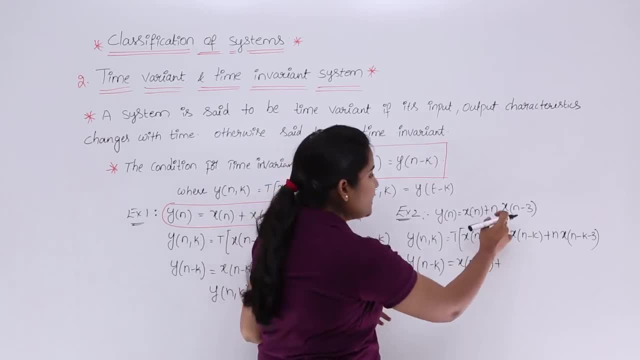 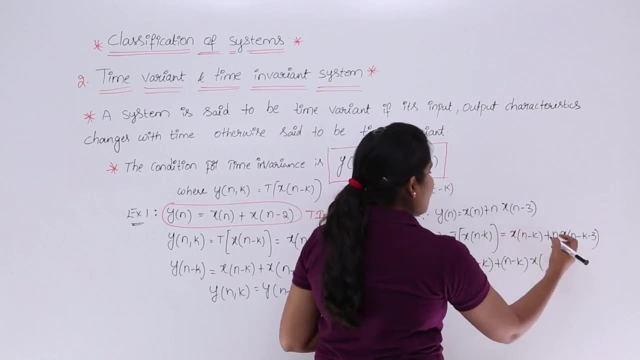 having n in the response, there you need to change. So here you are having n in the response. so here I am changing into n minus k, into x of. so here also I am having n means, so you need to substitute n minus k, minus 3.. 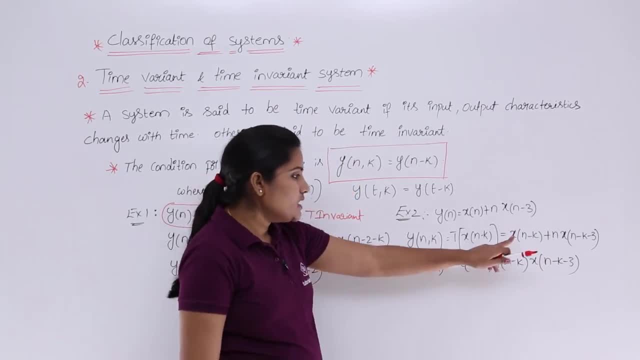 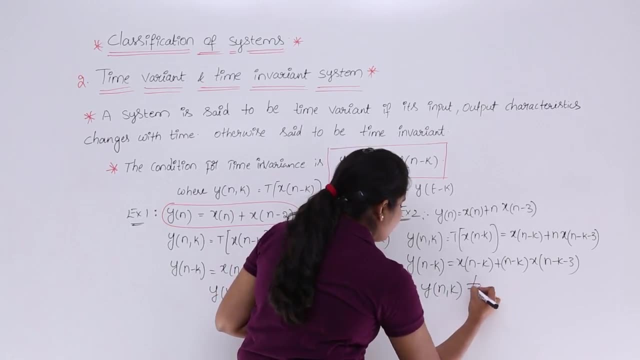 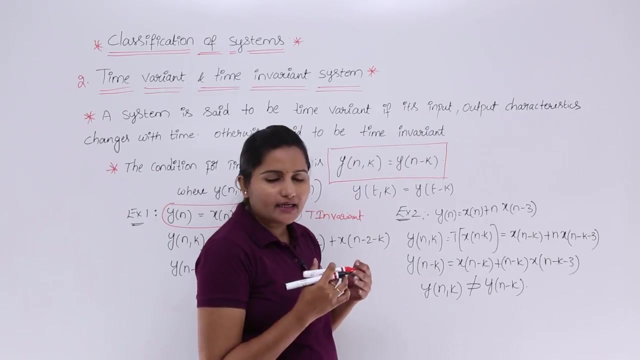 If you observe these two, input change and output change, So these two are not equal. so that is why in this case y of n comma k is not equal to y of n minus k. So in this case input is changing to output. that means characteristics of input output. 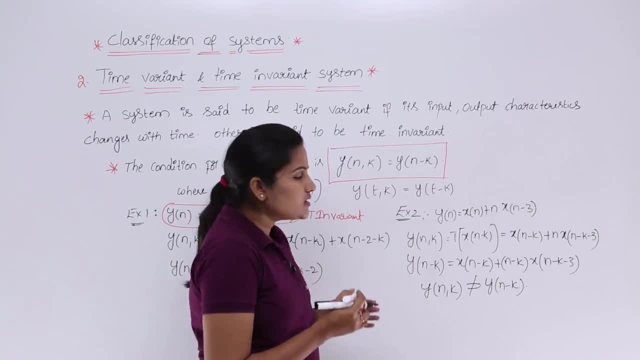 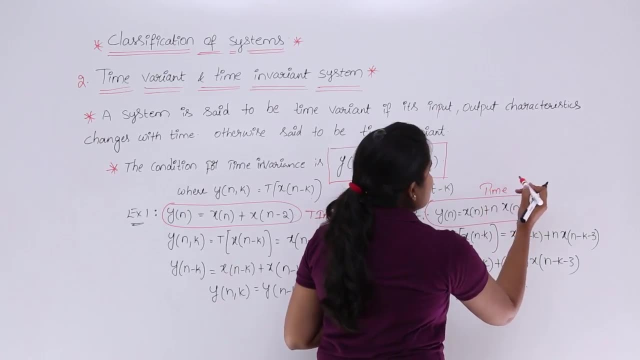 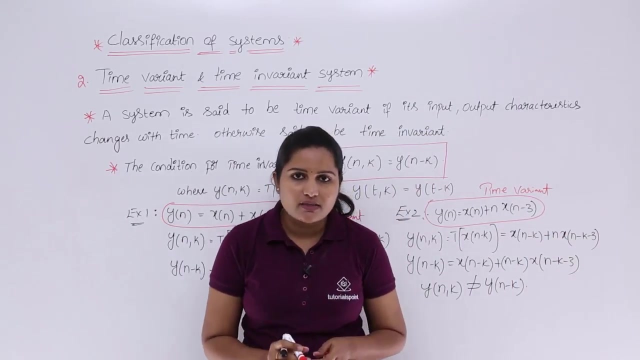 characteristics are going to change. So that means the system with this type of response is said to be time variant. So this is a time variant system response. Like this way we need to justify whether the system is time variant or time invariant.